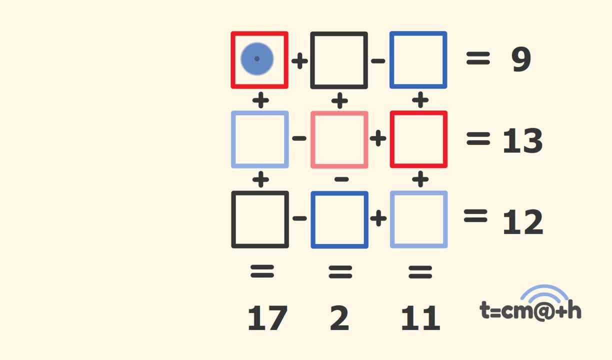 just to make it a bit easier to explain. So the red box we're going to call A, So this red box here is also A. The black box is B And this is also going to be B down here. This dark blue box is C, So this dark blue box is also C. 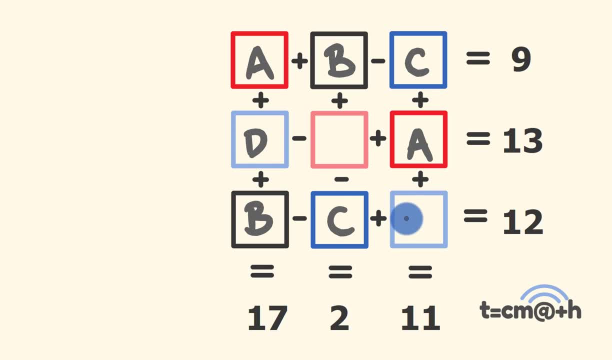 The light blue box is D, This one's also going to be D, And this one by itself we will call E. So there's a couple of things that we can see here. So, first off, you may have noticed that there's an A plus D here, and there's an A plus D here. 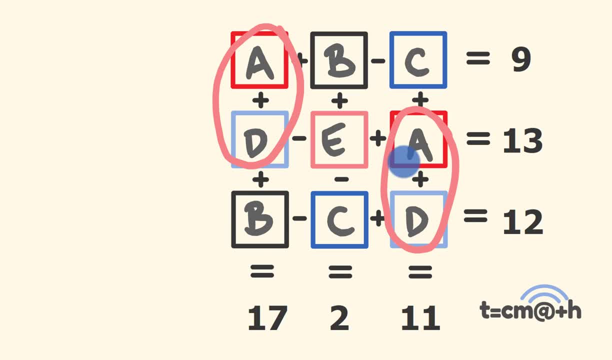 A plus D plus B here is equal to 17, and the A plus D plus C here is equal to 11.. So the difference between C and B would have to be 6. In fact, B is going to be the bigger one. so we can say the following is true: 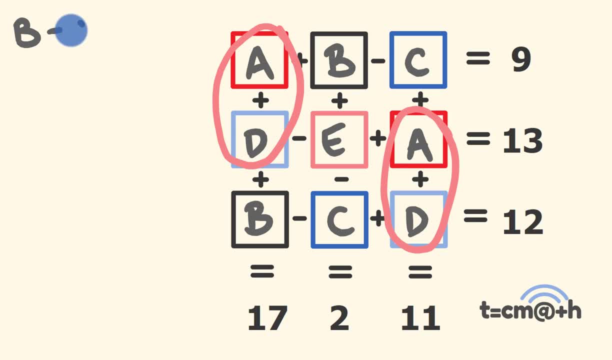 We can say that B subtract C is equal to the difference between 17 and 11, which is 6.. Now what you might notice is there There is a B subtract C just here, So we can substitute B, take away C with 6 here, because we know that value is 6.. 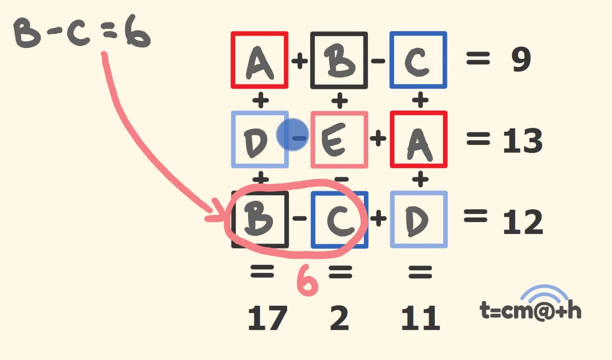 6 plus what number equals 12?. So we've worked out D right away. We know that D has to equal 6, because 6 plus 6 is equal to 12.. We can also substitute in the 6 value on the D over here. 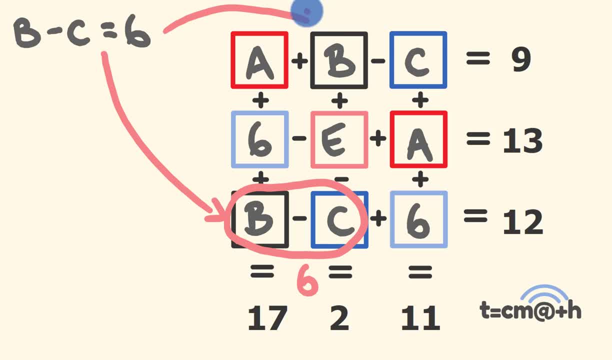 So let's do that. You also may notice, there is another B subtract C just here, So we can also substitute that in as well. We know that this is 6, so A plus 6 is equal to 9.. So we can work out what A equals. 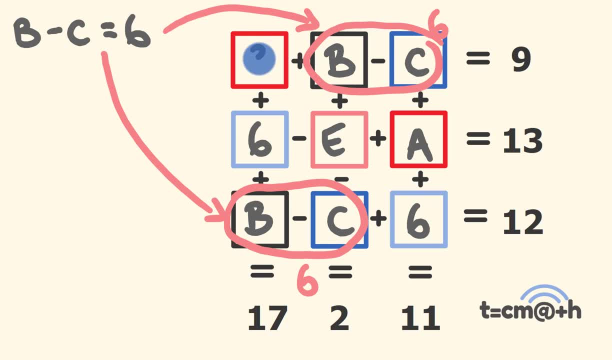 A, therefore, is going to be equal to 3, because 3 plus 6 is equal to 9.. We can also substitute this 3 value in down here, So it shouldn't be hard to work out the rest of these values. 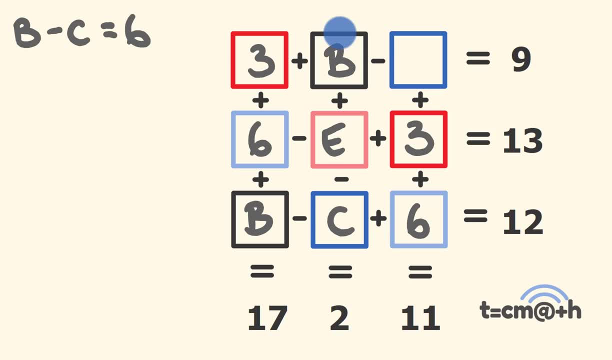 We can work out C here pretty simply, and we'll be able to work out this one here. So let's do this. What number plus 3 plus 6 equals 11?? Well, they'll have to equal 2.. And therefore this value here. 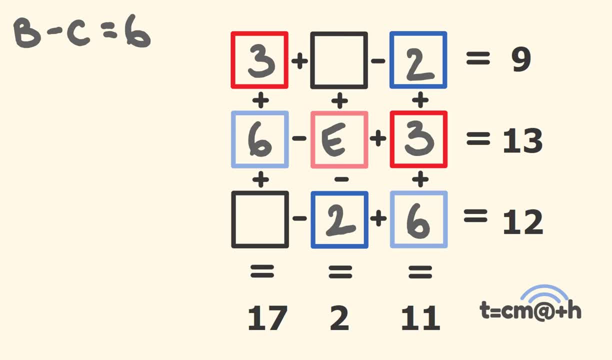 Is also 2.. We can now work out B, So let's work that out. What number subtract 2 plus 6 equals 12? That's going to be 8.. 8 take away 2 is 6, plus 6 is 12..